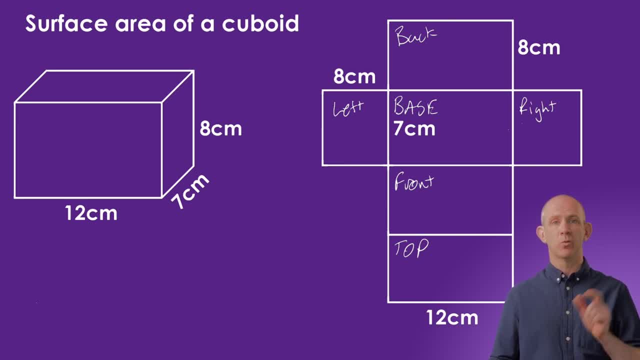 As this has matching sides, we can find one of each, add them together and then double it, Knowing there's a second side the same size to a total of all six sides. So the base will be 7 times 12, to give 84 centimetres. 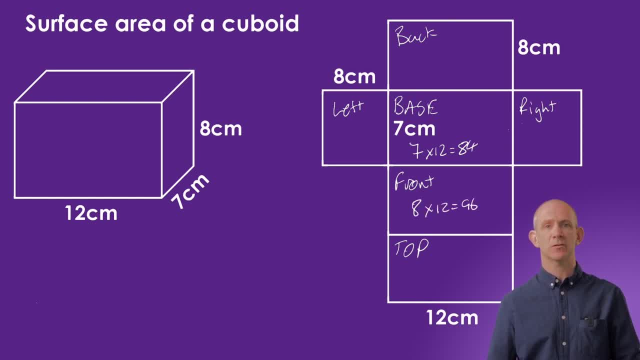 The front is 8 times 12,, to give 96 centimetres squared, And the left is 8 times 7, to give 56 centimetres squared. If we add these together, we get 236 centimetres squared, and multiply it by 2 to get 472 centimetres squared. 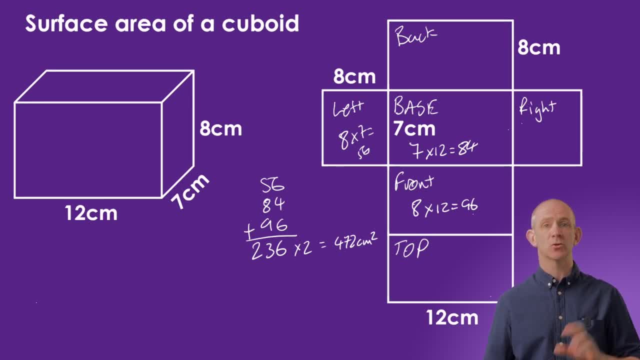 It's a good time to note that we're using centimetres squared with this measurement, because, although it's a 3D shape, we're looking at the two-dimensional shapes that cover the outside of it, As we'll see throughout this video. 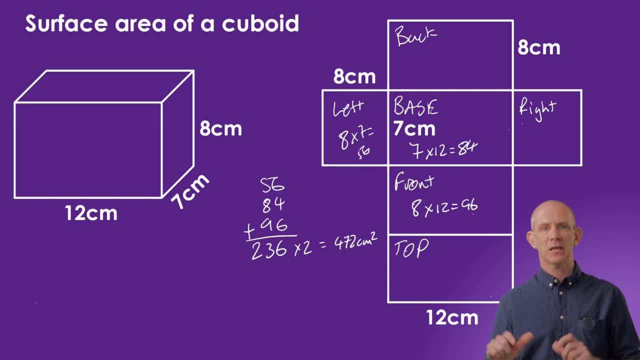 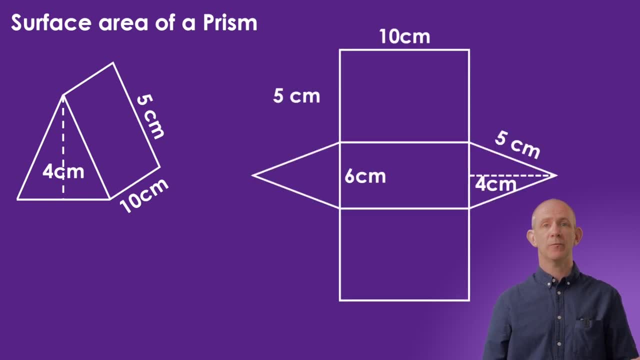 unfolding and getting the net of a cuboid is key to working out the surface area of any three-dimensional shape. In the next slide we have a triangular face prism. If we unfold it we'd have the following net: We'll label these to show the base, the left side, the right side, the front and the back triangles. 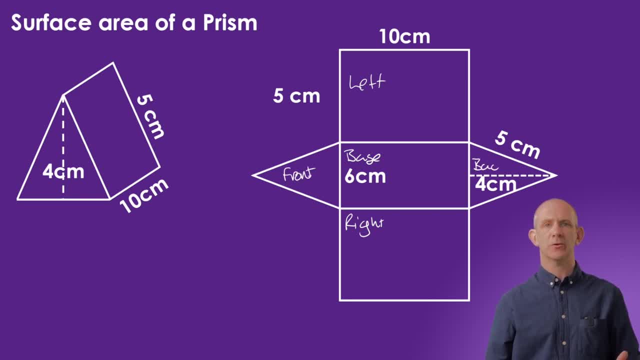 We need to calculate the area of each of these in order to add them all together to get the surface area. Let's start with the left rectangle: 10 times 5 would give 50 centimetres squared. The base rectangle 6 times 10 to give 60 centimetres squared. 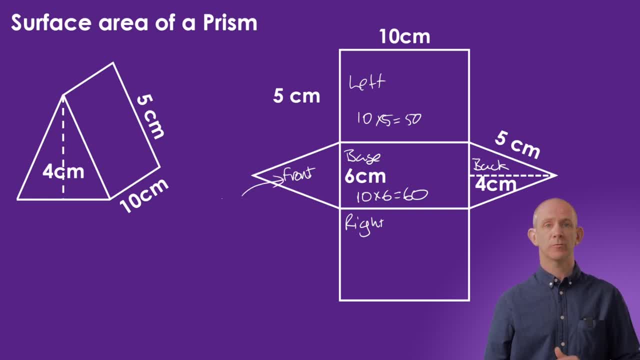 And now the front triangle: 6 times 4 divided by 2, to give you 12 centimetres squared. As we have two of the triangles, we can multiply that by 2 and get: 2 times 12 equals 24 centimetres squared. 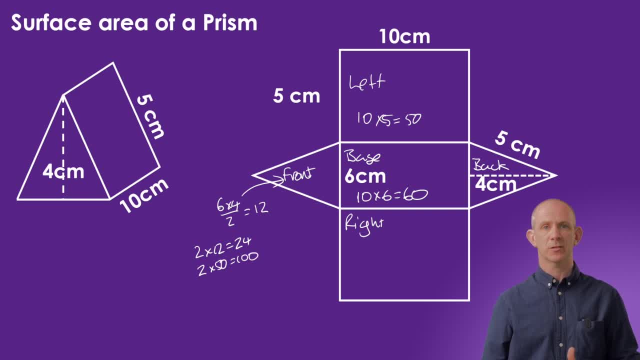 We also have two of the same rectangles which make the left and the right side. So 50 times 2 would give 100 centimetres squared. Now we can add all these sides together to get 184 centimetres squared, Which is the surface area for this shape. 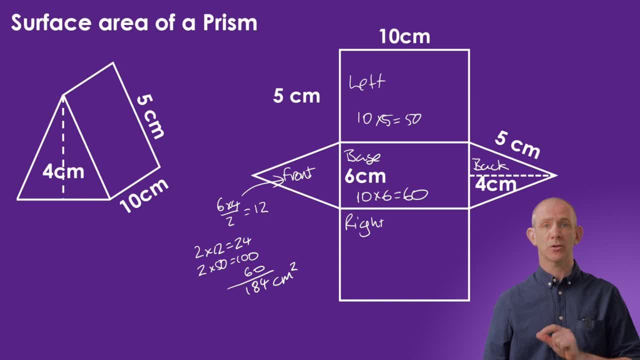 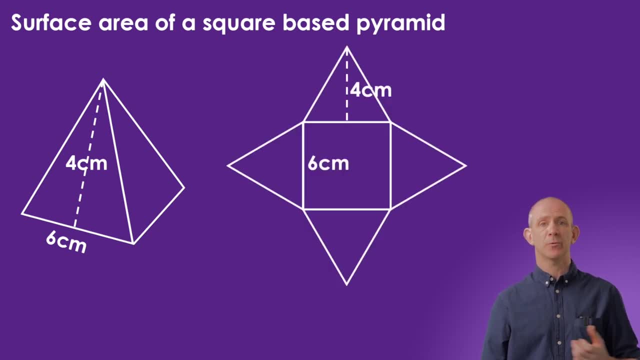 It's important to remember that we're just creating the net, calculating the area of each shape and then adding them together to get the surface area. Now we've got a square base pyramid And if we open it up, we get this net. 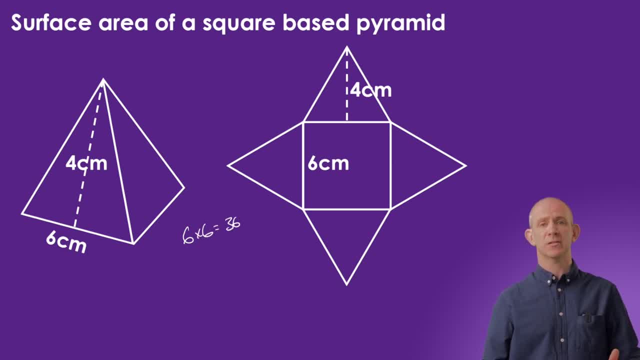 To calculate the area of the base, we should recognise it as a square and multiply 6 times 6 to give us 36 centimetres squared. Each of the triangles are the same height and base. We can calculate one of them and then multiply it by 4.. 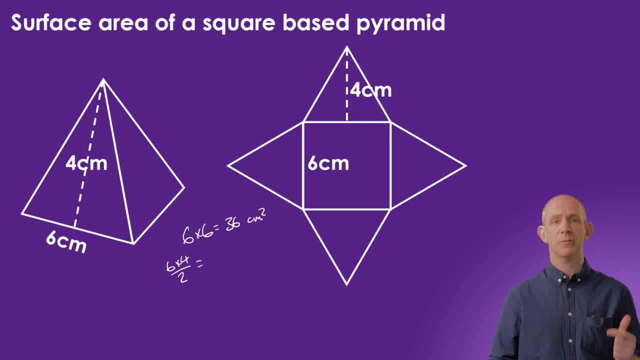 So 6 times 4, divided by 2, will give you 12 centimetres squared, And we can times that by 4 to get 48 centimetres squared. This is the total area for all of the triangular sides. If we add this to the base, we'll get the total surface area. 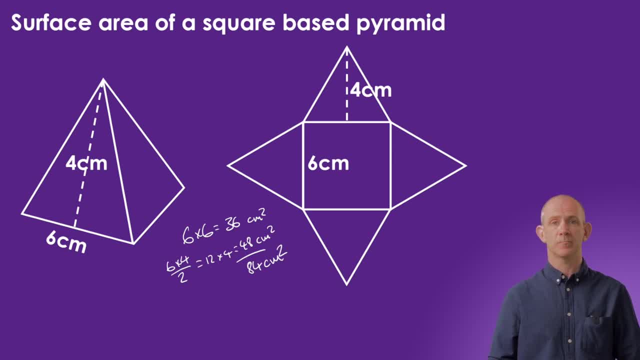 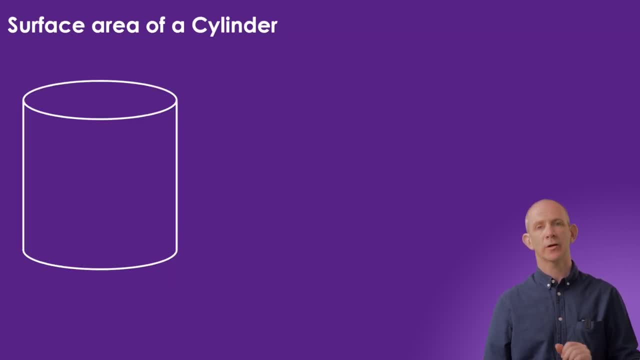 48 plus 36 will give us 84 centimetres squared, So we can double check that we've got all the sides of the shape and be confident we calculated it correctly. Next we're going to look at how to do this with a cylinder. 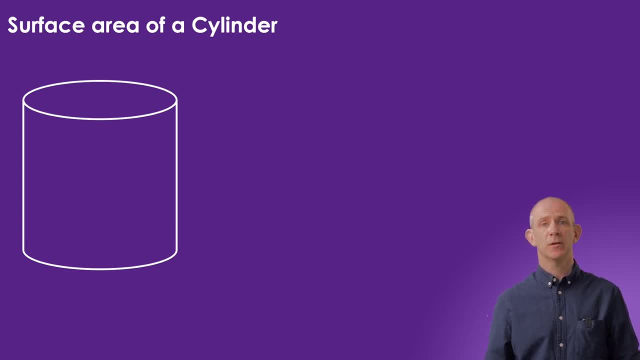 So we're going to find the surface area of this cylinder. If we were to open up this cylinder, we'd end up with two circles, one at the top, one at the bottom, and a very long rectangle. The reason for the length of this rectangle is it will be just over 3 times the diameter of the circles, as it will be the same length as the circumference of the circles at either end. 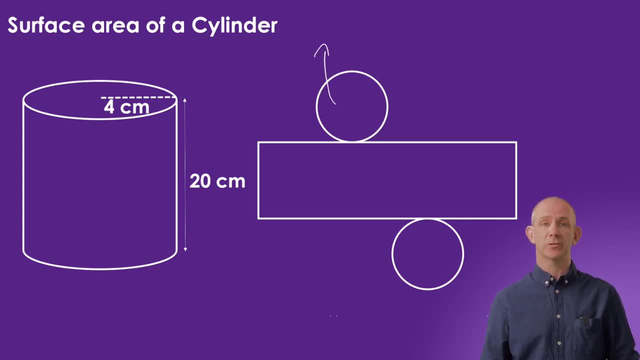 The width of the rectangle is going to be the same as the height of the original cylinder. So let's start by creating the area of one of the circles, And we know that the area of a circle is pi times the radius squared. So pi times 4 squared will give us 16 pi. 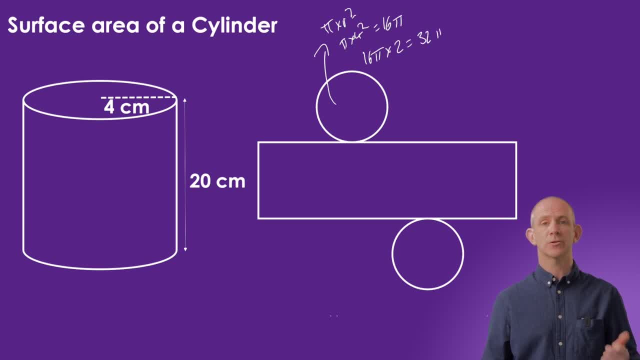 We'll times that by 2, as there's two circles to give us 32 pi or 100.53 centimetres squared. After we press the SD button, This will be the area for both of the circles. Now to calculate the area of the rectangle. 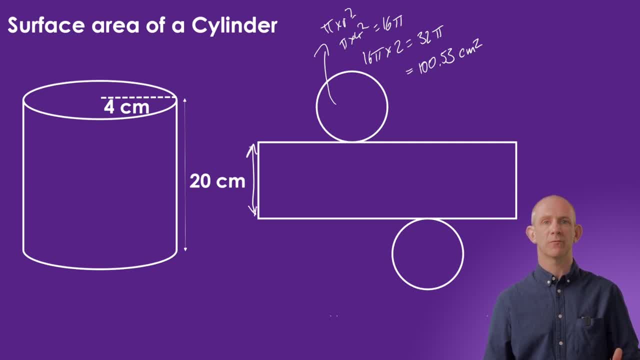 In order to do this, we need the length, which we know is equal to the circumference of the circle, So we can calculate it as pi times 8, which is the diameter, Which will give us 8 pi To get the area of the shape. we can then do 8 pi times 20 centimetres, which is the width of the rectangle. 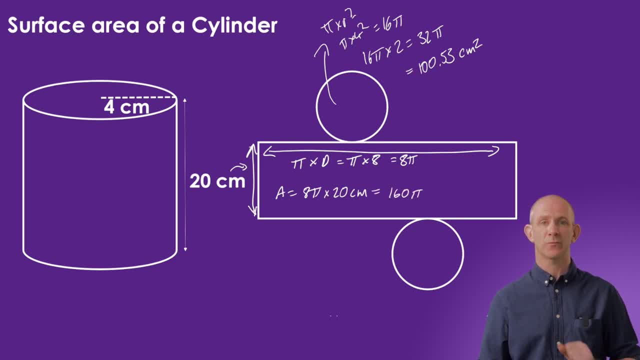 Which will give us 160 pi or 502.65 centimetres squared. If we add these two totals together, we get an overall total of 603.19 centimetres squared. I've rounded this to two decimal places because we haven't specified the degree of accuracy. to put it to: 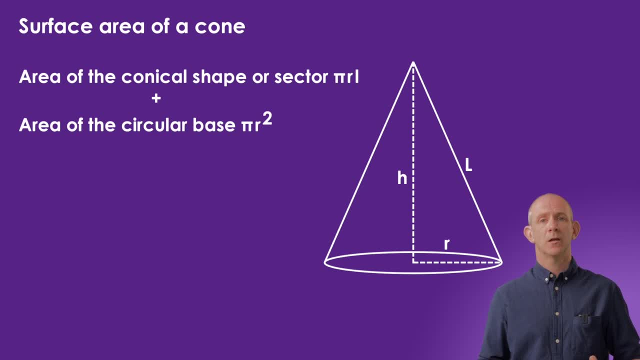 And if I'm in doubt I always just round it to two decimal places. Lastly, we're going to find the surface area of a cone And we've been given the formula for finding the area of the conical shape and then told to add it to the area of the base to get the total surface area.